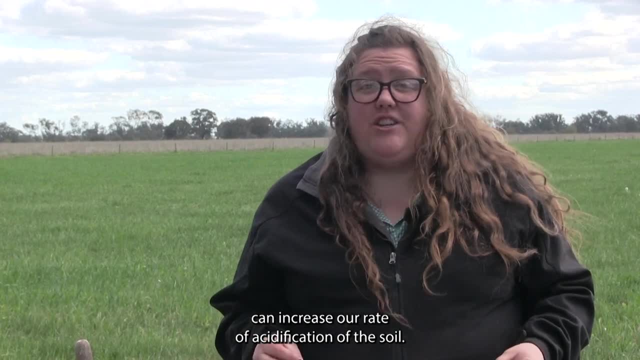 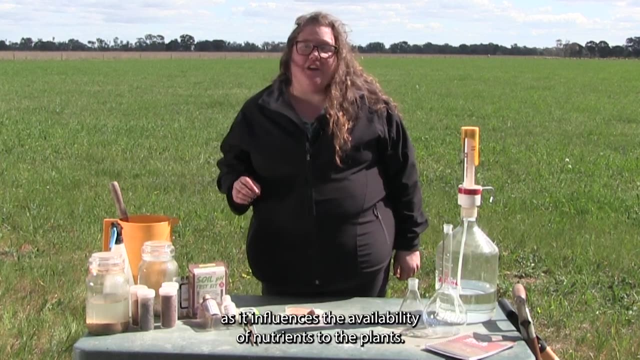 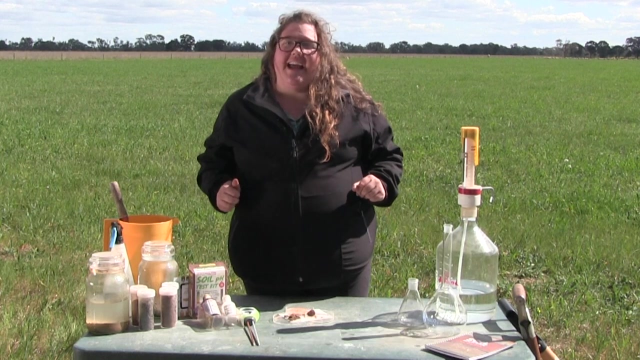 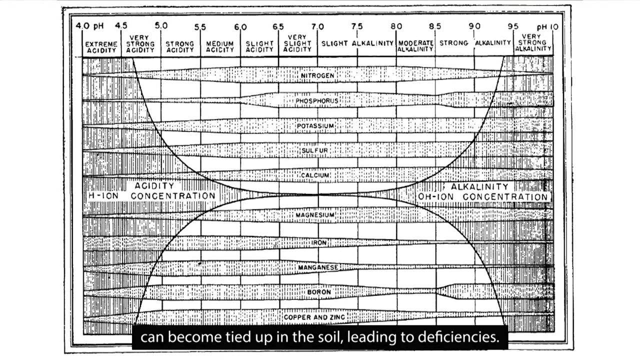 some farming activities can increase our rate of acidification of the soil. Soil pH is important to understand and manage as it influences the availability of nutrient nutrients to the plants. If the soil is too acidic or too alkaline, some nutrients required for good crop plant growth can become tied up in the soil, leading to deficiencies and 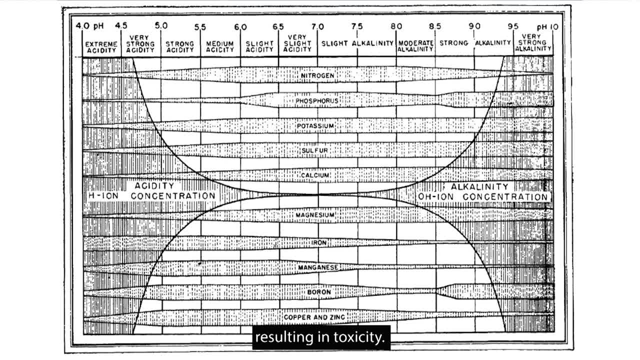 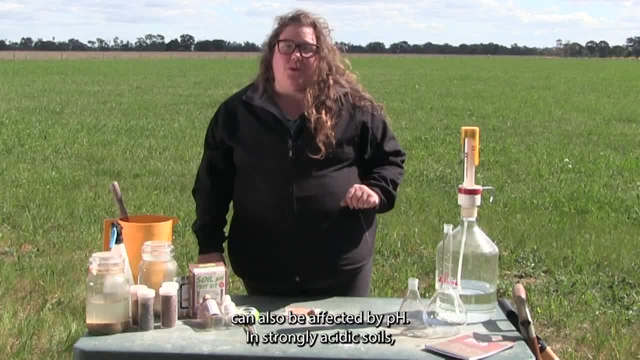 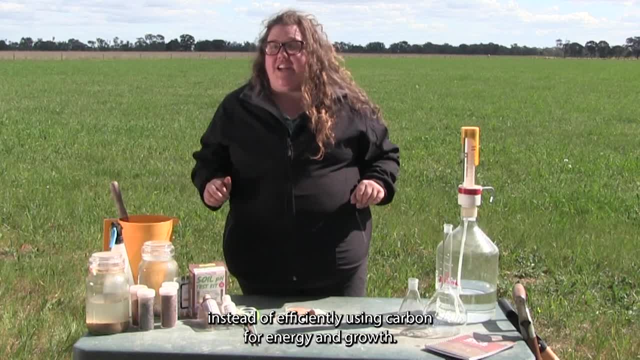 some that we don't want in the soil can be released, resulting in toxicity. Soil microbial activity can also be affected by pH. In strongly acidic soils, microbes direct more of the carbon consumed into respiration activity Instead of efficiently using carbon for energy and growth. this results in soils having an 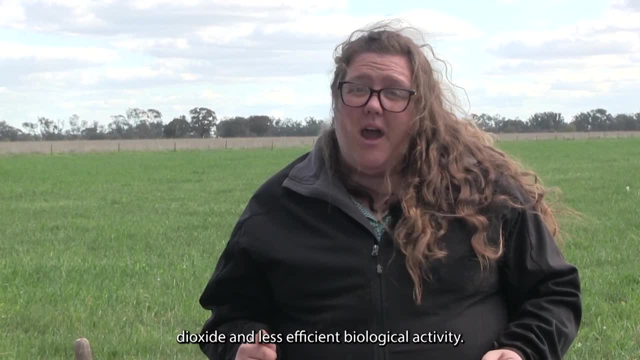 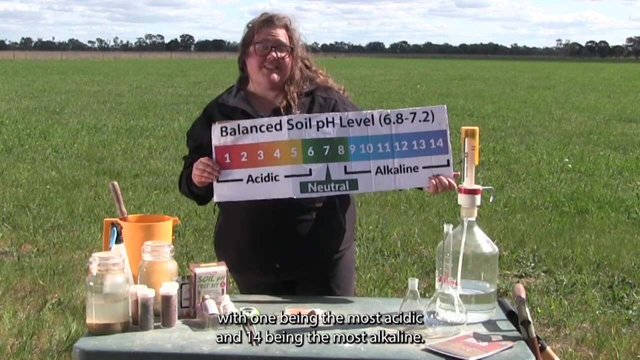 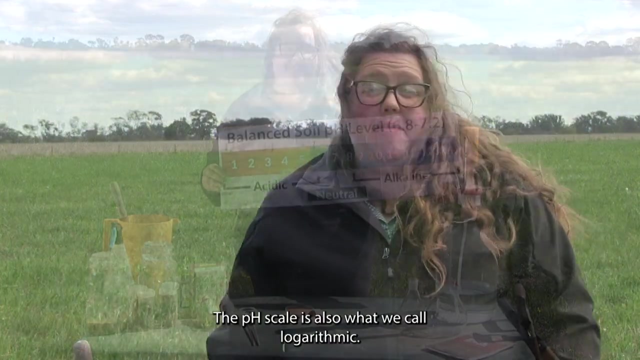 increased release of carbon dioxide and less efficient biological activity. The pH scale goes from 1 to 14, with 1 being the most acidic and 14 being the most alkaline. A pH of 7 is considered neutral. The pH scale is also what we call logarithmic. I know high school maths. 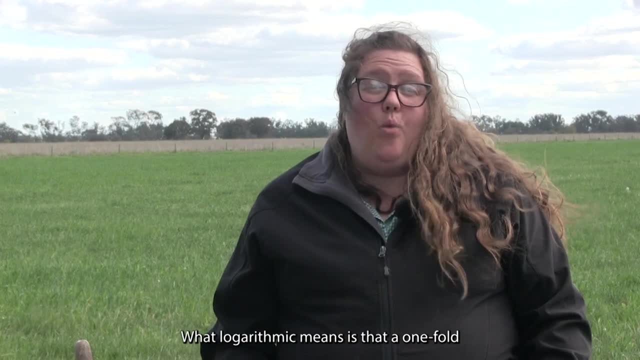 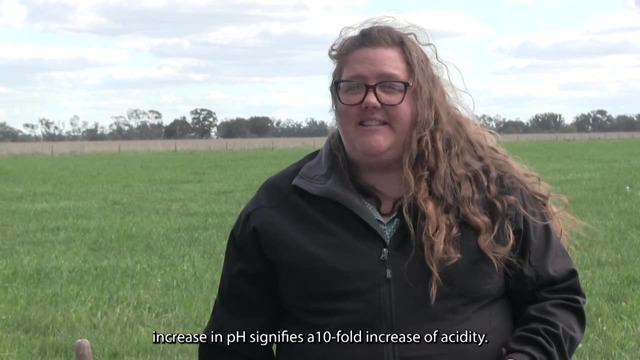 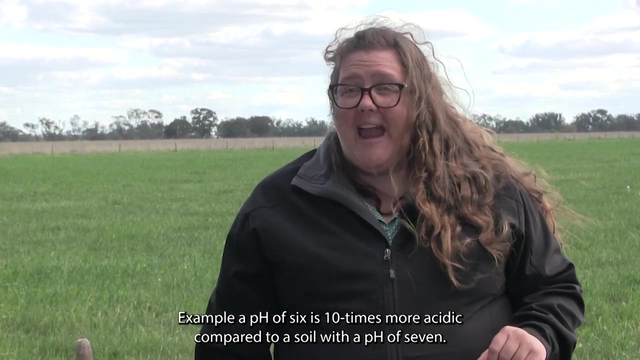 But it's coming in useful here. What logarithmic means is that a one-fold increase in pH signifies a ten-fold increase of acidity. For example, a pH of 6 is 10 times more acidic compared to a soil with a pH of 7.. 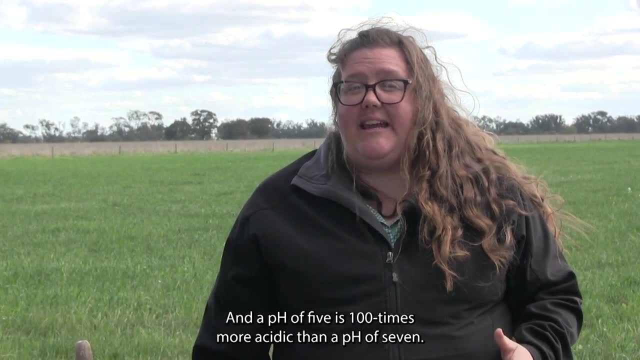 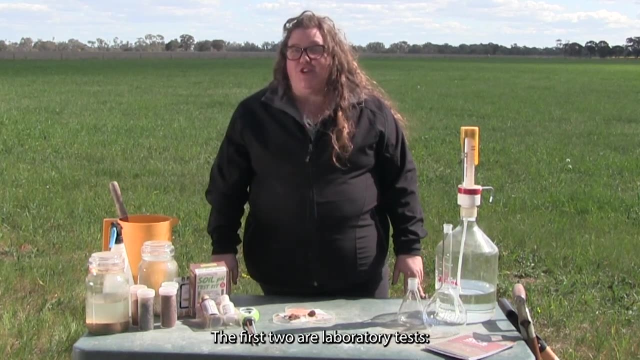 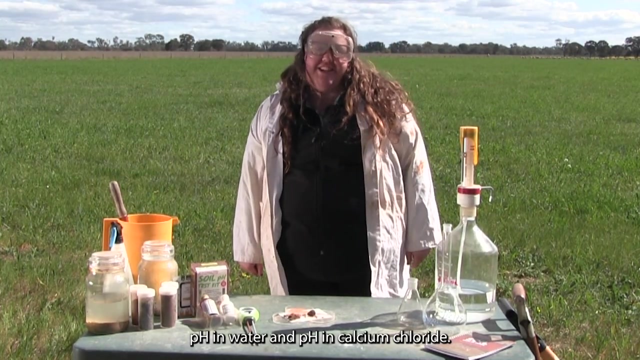 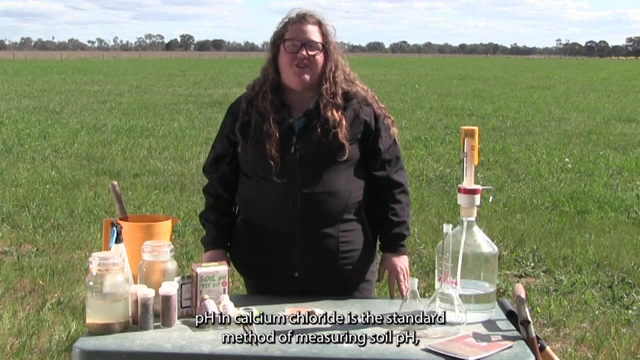 And a pH of 5 is 100 times more acidic than a pH of 7.. pH can be measured in four main ways. The first two are laboratory tests: pH in water and pH in calcium chloride. pH in calcium chloride is the standard method of measuring soil pH, reflecting what the 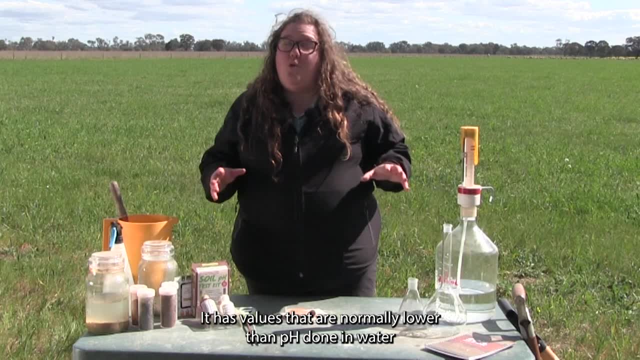 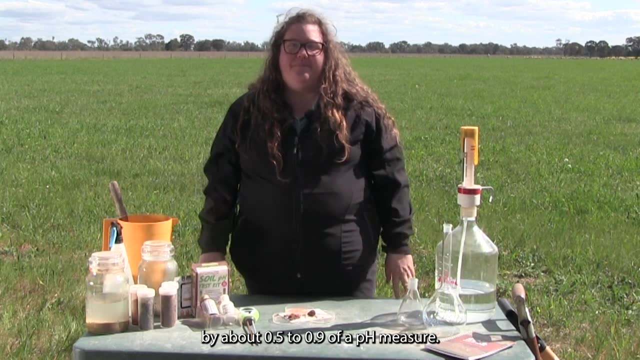 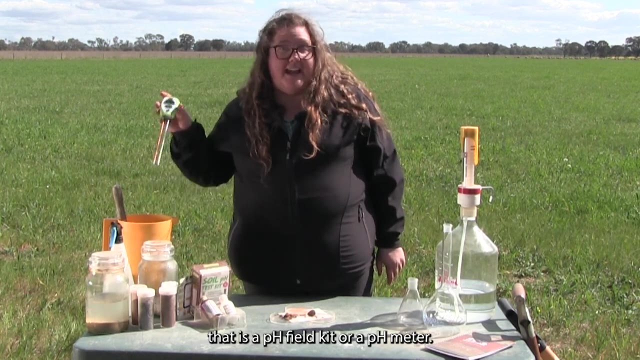 plant experiences in the soil. It has values that are normally lower than pH done in water by about 0.5 to 0.9 of a pH measure. The final two methods are used in the field, That is, a pH field kit or a pH meter. 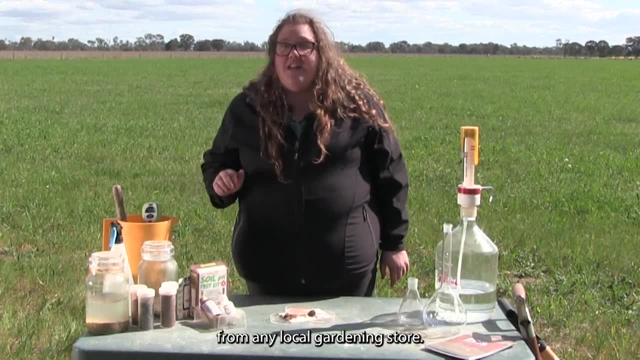 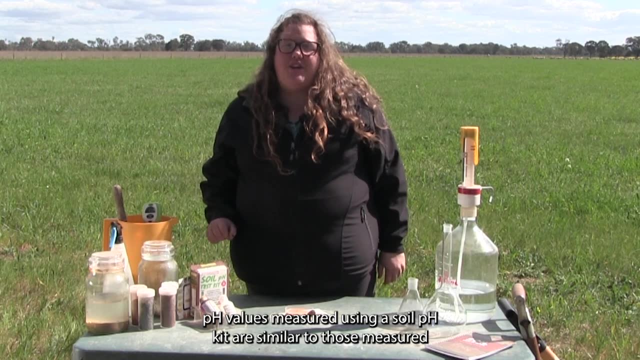 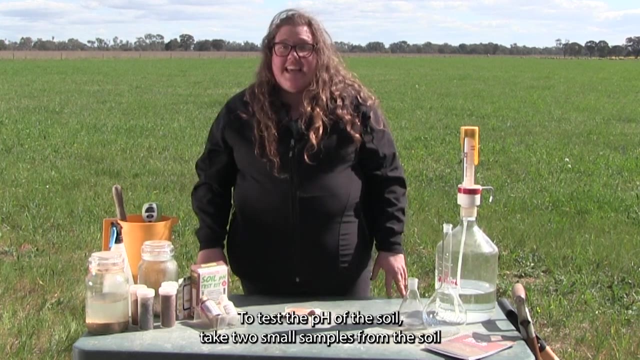 We will use a kit that can easily and cheaply be purchased from any local gardening store. pH values measured using a soil pH kit are similar to those measured in water and accurate to about plus or minus 0.5 of a pH unit. To test the pH of the soil, take two small samples from the soil from the side of the 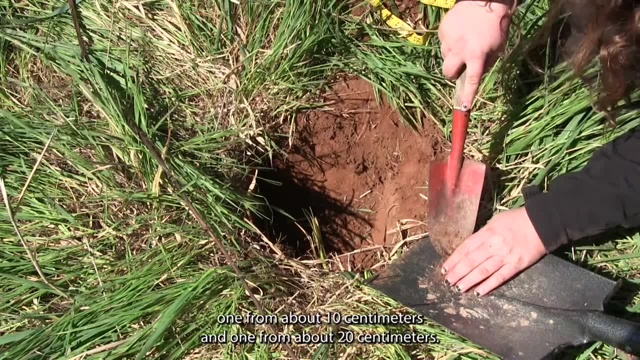 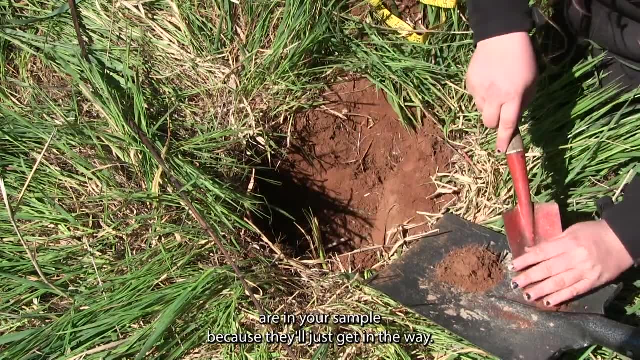 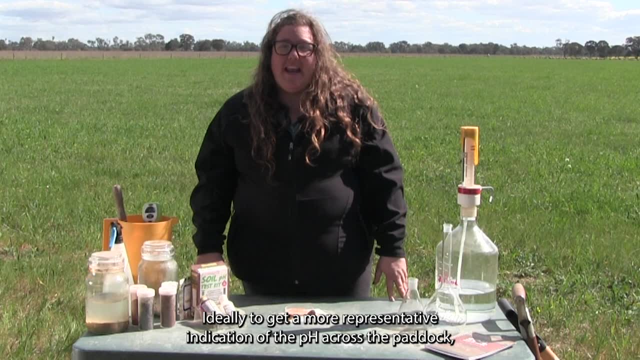 small hole dug, One from about 10 centimetres and one from about 20 centimetres. Make sure that no plant material or stones are in your sample, because they will just get in the way. Ideally, to get a more representative indication of the pH across the paddock, you would take 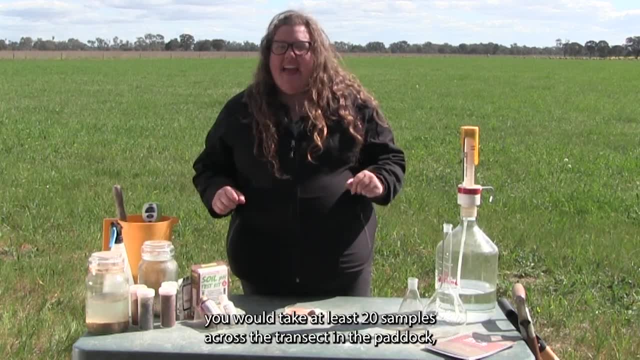 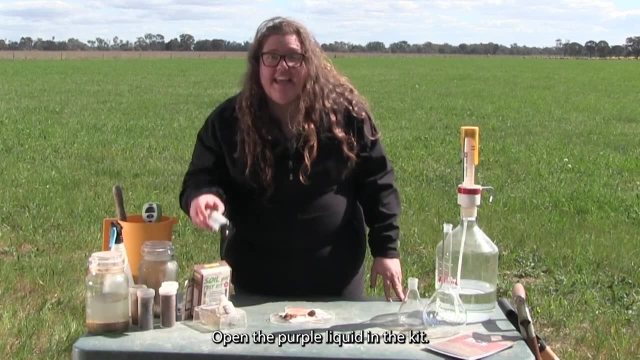 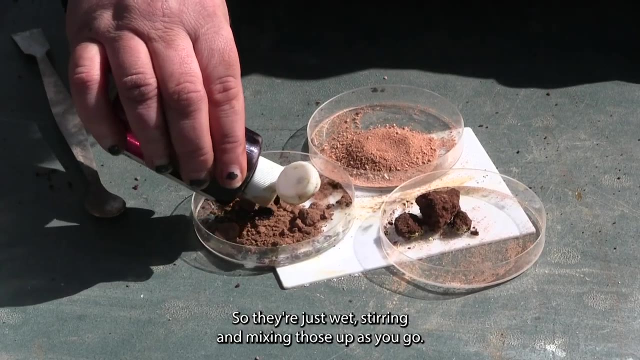 at least 20 samples across the transect in the paddock. Mix them together thoroughly and then sub-sample from there. Open the purple liquid in the kit- This is the indicator dye- And cover the soil samples. so they're just wet, Stirring and mixing those up as you go. 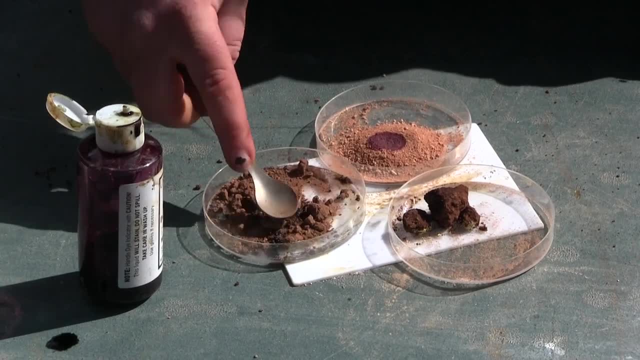 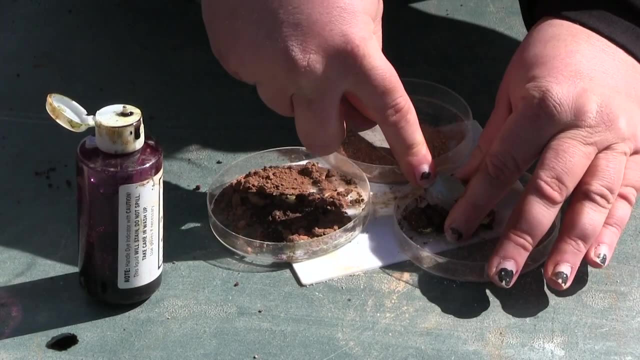 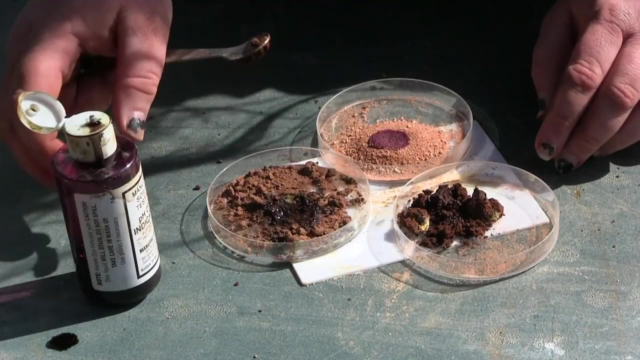 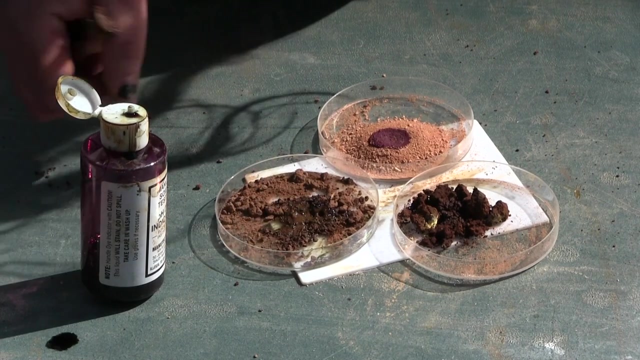 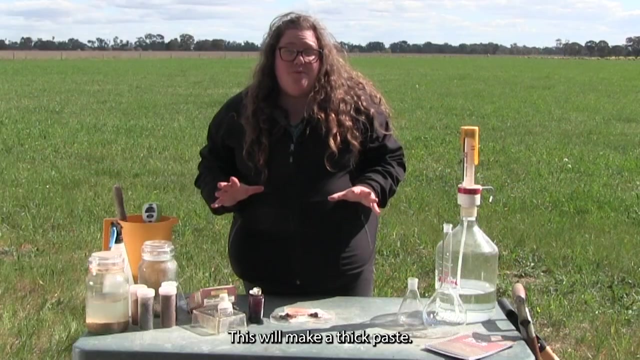 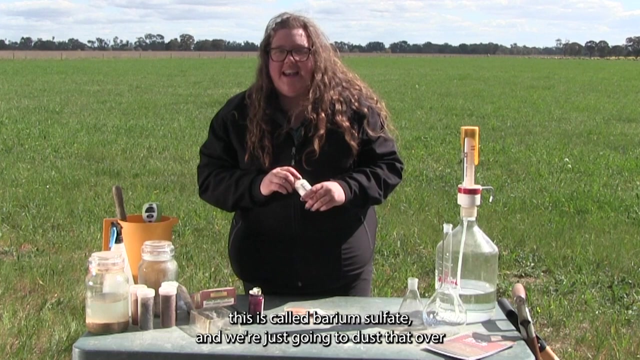 This will make a thick paste. Once you have your thick paste, take out the white powder, and this is called barium sulfate, and we're just going to dust that over the soil, just enough to cover and bring up the 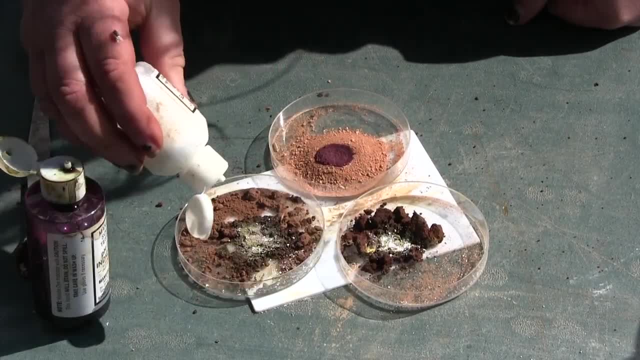 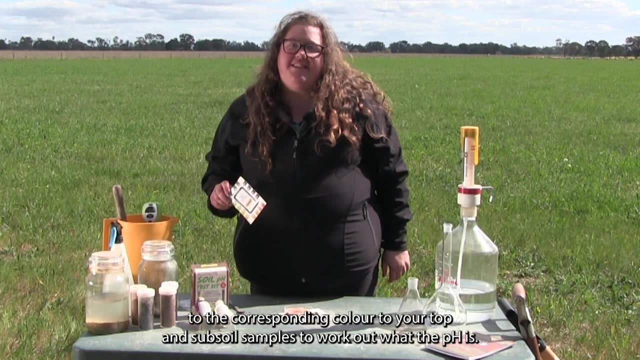 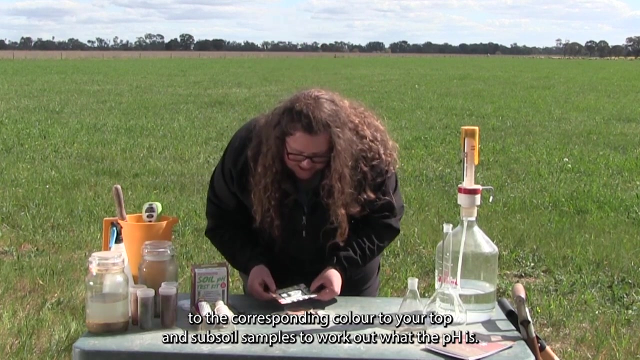 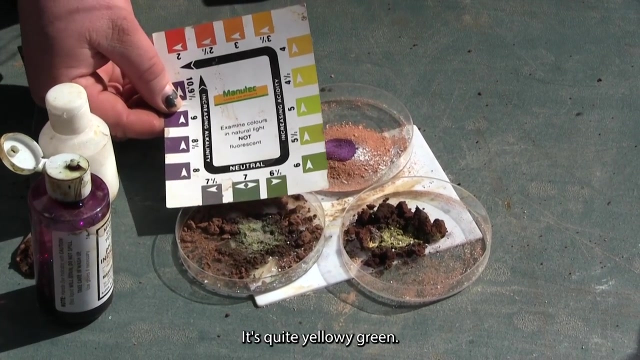 soil colour. Now you can take out the colour chart that's in the kit and match that to the corresponding colour to your top and subsoil samples to work out what the pH is. Here we can see that we have a pH of about five and a half. it's quite yellowy green. 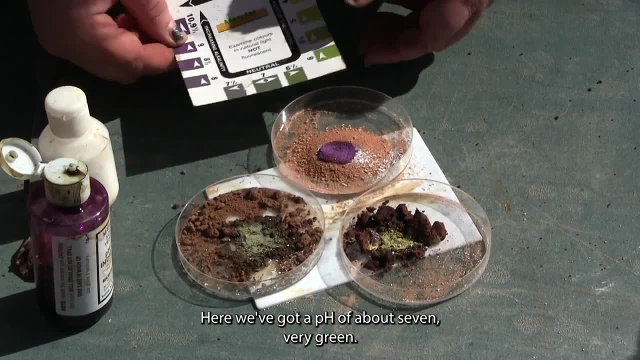 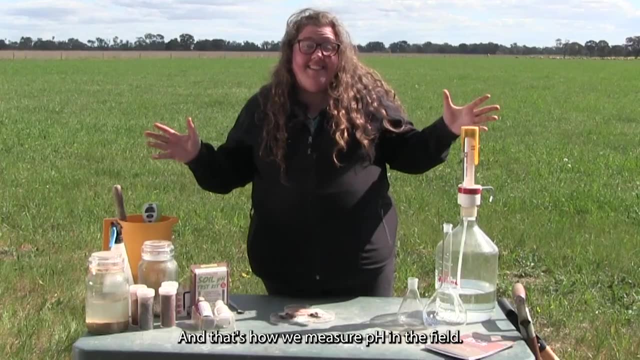 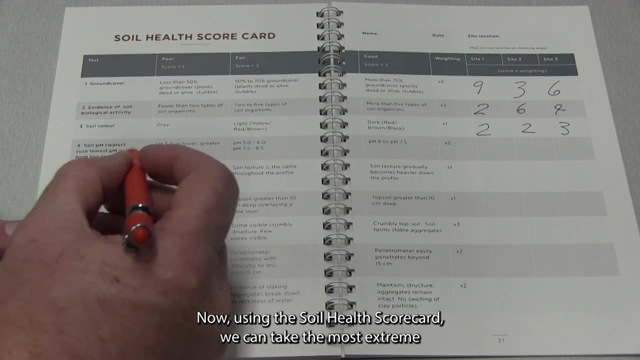 Here we've got a pH of about seven- very green- And here we've got an alkaline soil, a pH of about nine because it's purple. And that's how we measure pH in the field. Now, using the soil health scorecard, we can take the most extreme pH value and assess. 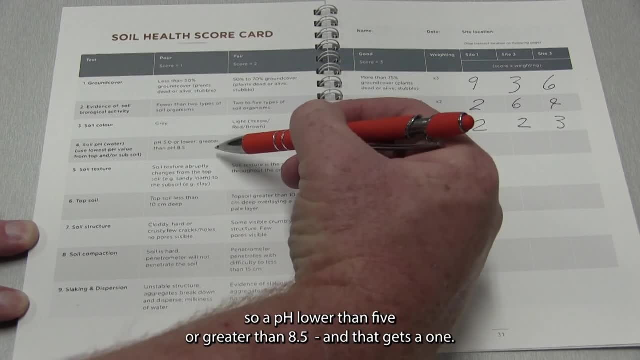 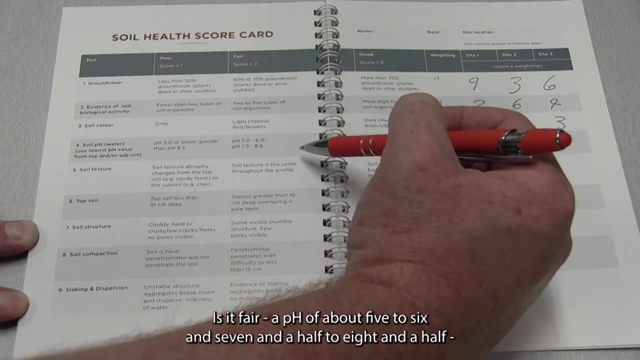 if the soil pH is poor. so a pH lower than five or greater than 8.5, and that gets a one, Is it fair? A pH of about five to six and seven and a half to eight, Eight and a half, and that gets a score of two. 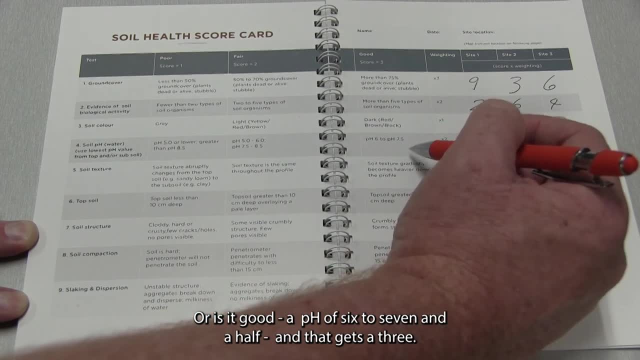 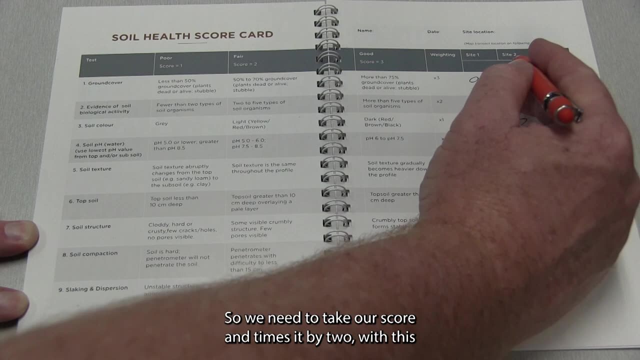 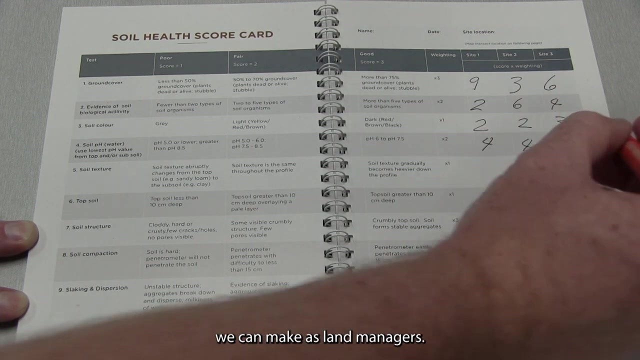 Or is it good A pH of six to seven and a half and that gets a three? Soil pH has a weighting of two, so we need to take our score and times it by two, with this soil health factor being moderately influenced by decisions we can make as land managers. 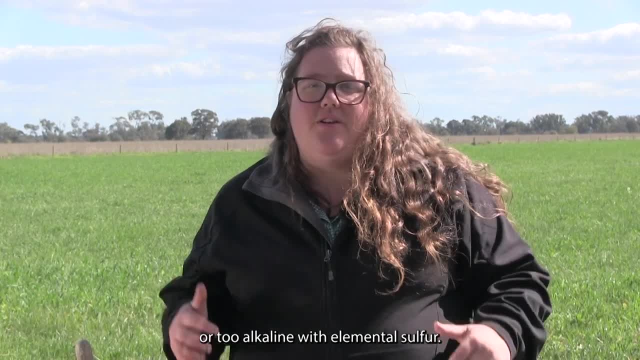 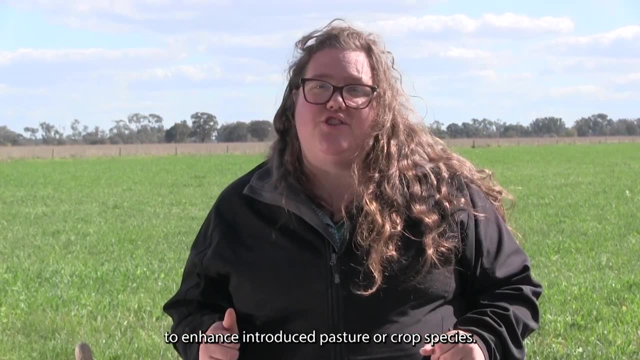 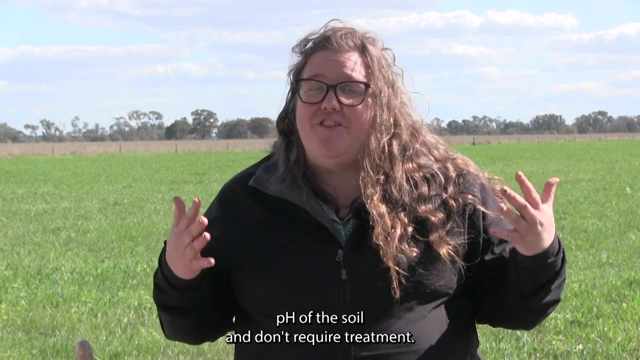 Soil that is too acidic can be treated with lime, or too alkaline with elemental sulphur. Keep in mind, though, Your pH should only be changed to enhance introduced pasture or crop species. Native grasslands are perfectly adapted to the natural pH of the soil and don't require treatment. 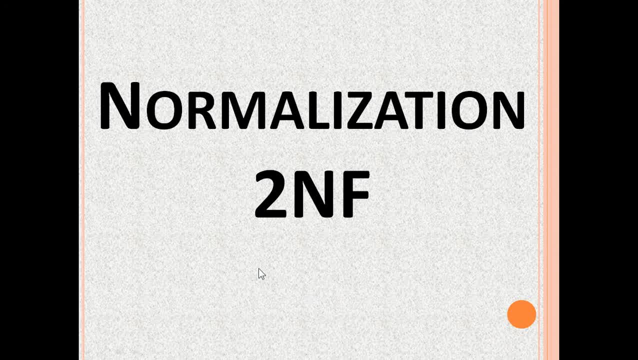 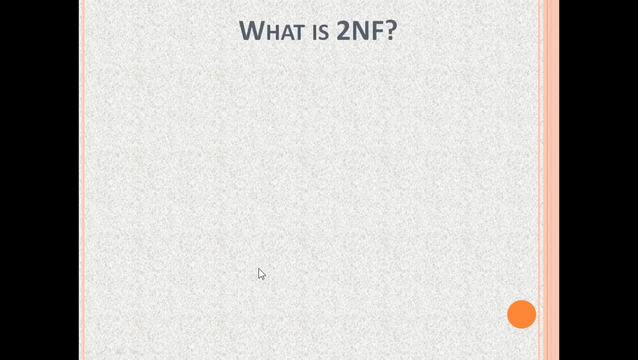 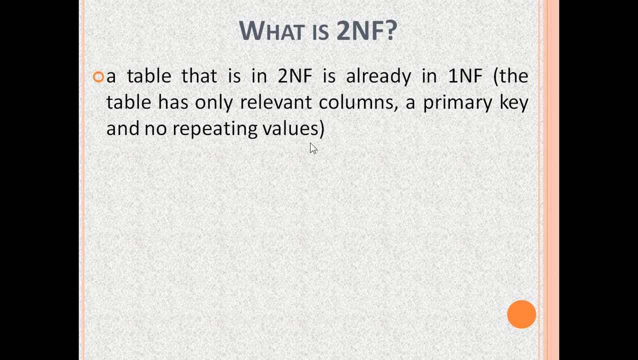 Hello and welcome to this second normalization tutorial for beginners. In this video we will learn about the second normal form. What is 2NF? A table that is in 2NF is already in 1NF, Meaning the table has only relevant columns, has a primary key and no repeating values. 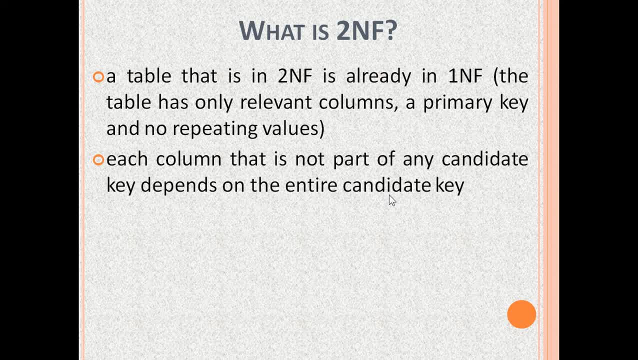 Now, candidate key means one or more columns whose value is unique in every row To be in 2NF. each column that is not a part of the candidate key depends on the entire candidate key. We will see multiple examples of this shortly. 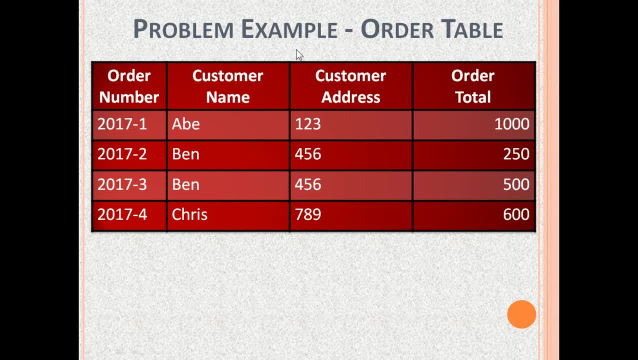 Now let us see some examples of tables that are not in 2NF and how to normalize them to 2NF. This is the order table. Its columns are order number, customer name, customer address and order total. In this table, the only candidate key is order number that is unique in every row of the table.